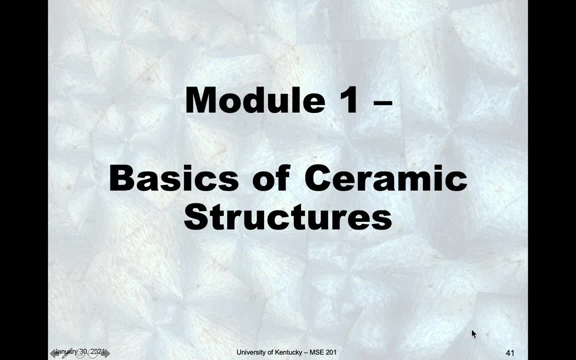 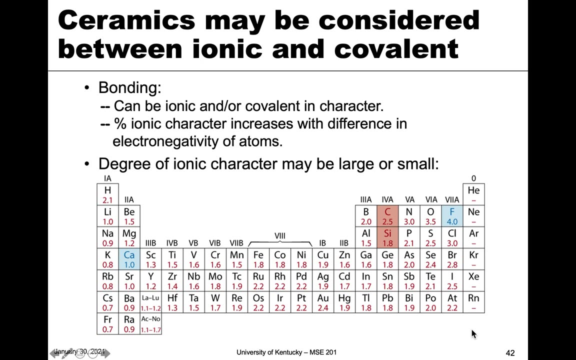 Alright, in this module, today's lectures, we are going to talk about ceramic structures and we'll start with kind of some of the basics of these ceramic structures. Alright, so, as we talked about with bonding, ceramics can have ionic and covalent and they're usually considered some mixture of the two. We 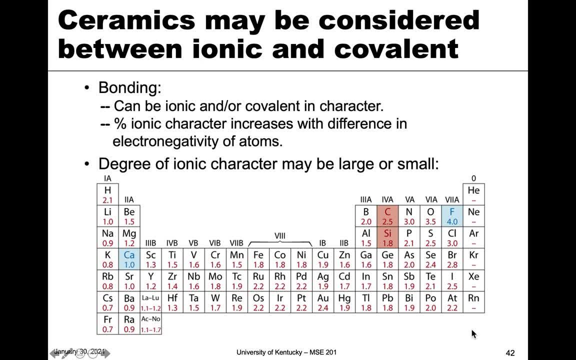 looked at that percent ion character equation and that's all due to the differences in electronegativity And so the two we can look at here. calcium fluoride is a ceramic and we have a pretty large difference- three on this absolute scale- here, Whereas if we're looking at something like silicon, 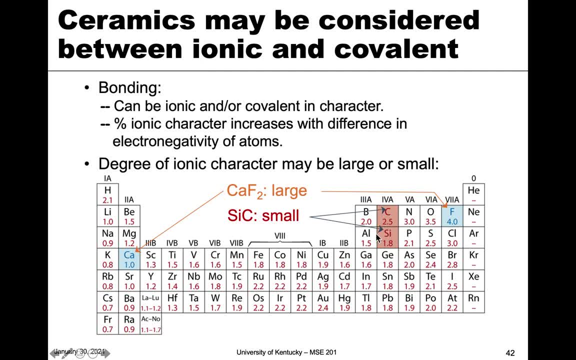 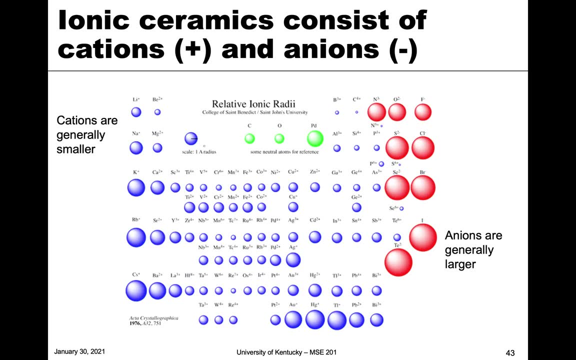 carbide, there's a much lower- less than one- difference in the electronegativity values. So that is going to dictate the type of bonding that we have and the type of structure. But we're gonna start with ionic, because ionic can be a little easier to describe And so we know that we form ions. 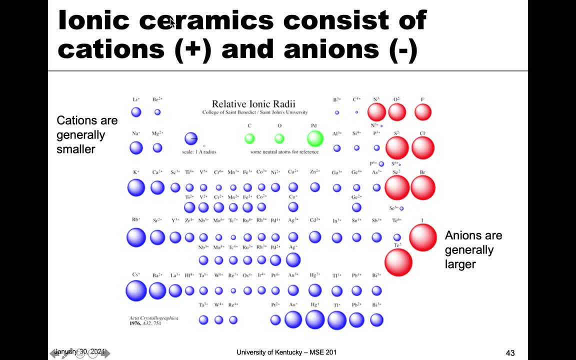 cations and anions. and so, just as a refresher, cations are those positively charged ions, so basically the metals, and so they're kind of highlighted in blue throughout here. And then the anions are the negatively charged ions, and those are highlighted in red and those tend to be the non-metals, And so 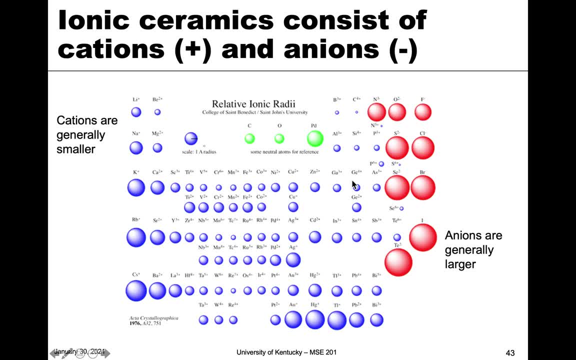 this chart here, which is in the shape of the periodic table, shows you the relative ionic size. So if we kind of compare to their, to their kind of base neutral, then removing electrons tends to make things smaller, And so you can see carbon here. 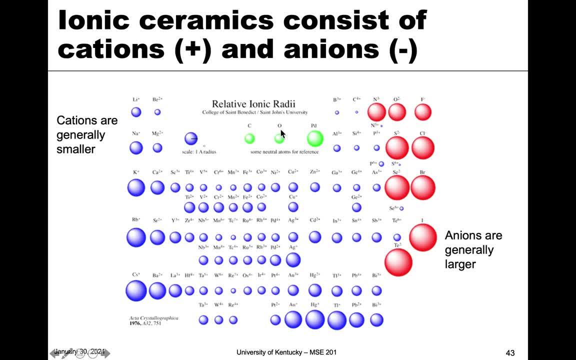 and if we remove electrons from carbon, you can see it gets smaller. And so cations- we generally think of the smaller of the two- And then anions- we're adding electrons. So if we compare, for example, oxygen to minus, we're adding two. 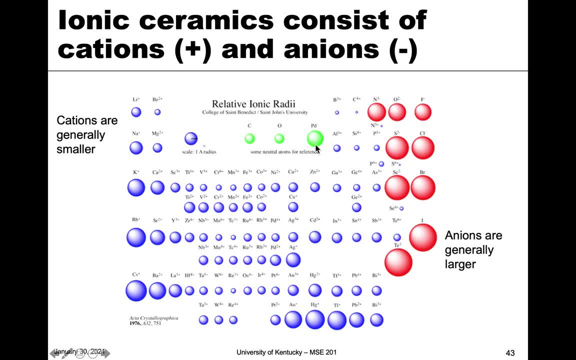 electrons. If we compare it to the neutral atom for reference, we can see that it's gotten bigger. So we generally say that anions are larger of the two, And so this is going to be important for how we think about the structures of ionic ceramics. So you want to make sure. 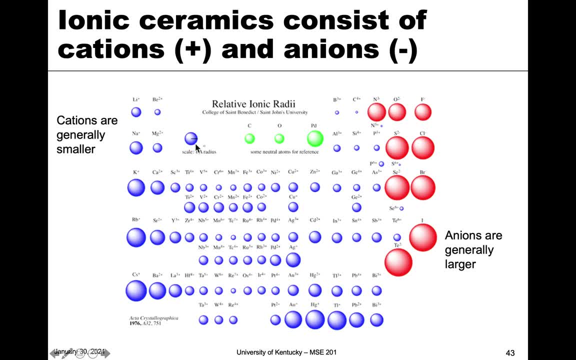 that you remember, anions are generally larger, cations are generally smaller But, as you might be able to tell, there's going to be certain cases where, if you pick a really big cation, like cesium, and a really small one, like 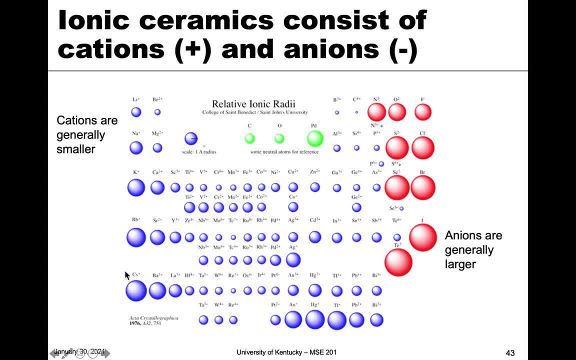 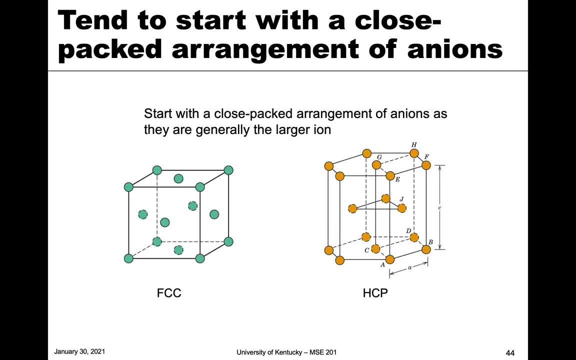 chlorine, then that can be inversed. Or if they're very similar in size, cesium and chloride, Okay, so because the anions are bigger, when we're looking at ionic ceramics, what we tend to think of as the anions forming one of the close-packed 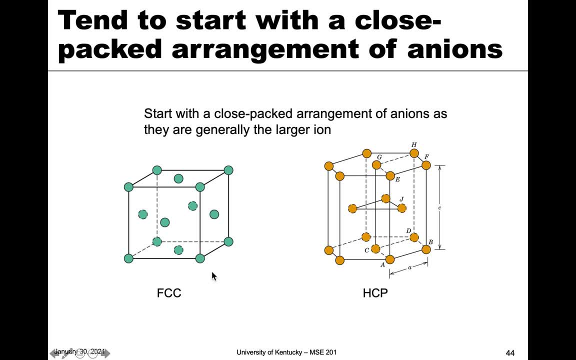 arrangements. And so those two that we talked about in the metallic structures, FCC and HCBs- right, They had the same atomic packing factor. They're the closest packing you can get for similar sized ions. So for ionic ceramics, we're going to basically think of most of these. 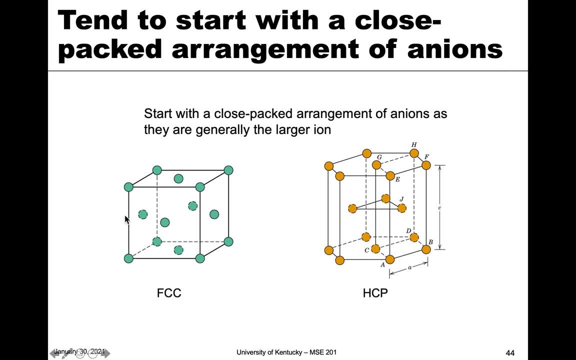 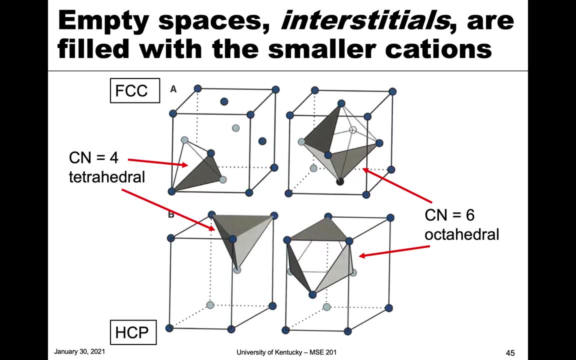 structures as the anions being in one of these two arrangements. And so, basically, how we approach it is we start with one anions in either this or this arrangement, and then we think about where those cations would go, And where we find they go is, as you imagine, the empty spaces, right? So? 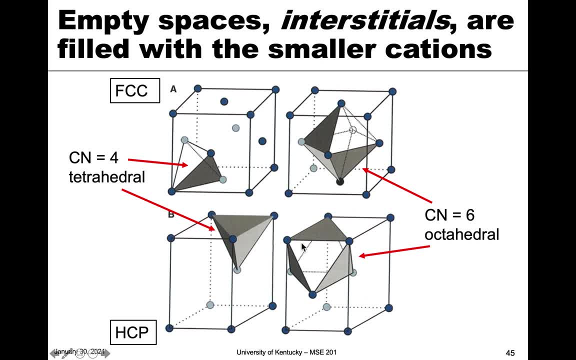 this is FCC up here. This is another kind of representation of HCP, not showing the hexagonal form of it, but still showing the structure. What we find is that these empty spaces in these structures are located in specific places, So located here, for example, or right in the middle. 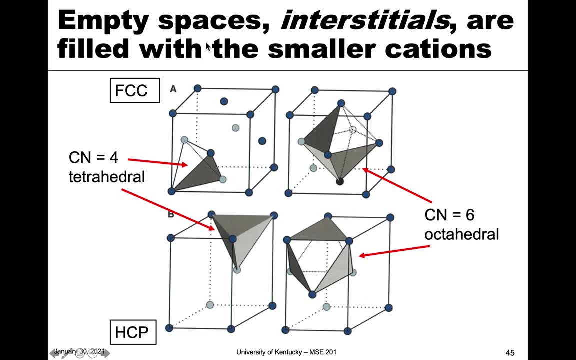 of the cation And these empty spaces. we don't call them empty spaces, we call them interstitials. Basically, if you kind of think about that name, it's in between the spaces, And so this is where we fill the. 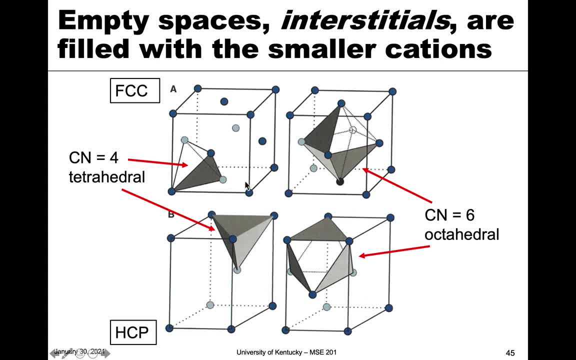 smaller cations. So basically we have a close packed arrangement of anions that are large and then we fill in the empty spots of the structure with cations. I do want to make a mention here is that once we put the cations in these empty spaces, that doesn't mean we maintain. 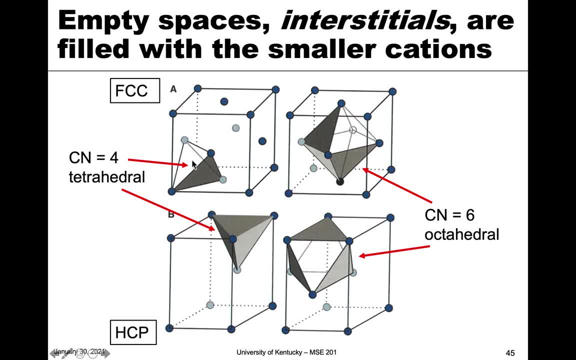 FCC structure or that things stay the same. cations are not actually the size of these empty spaces. they actually kind of blow them up a little bit. they're too large for these spaces And so they tend to expand the structure and still is still different. We don't have the same kind of. 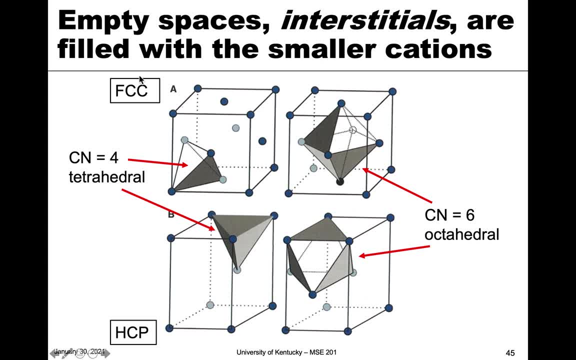 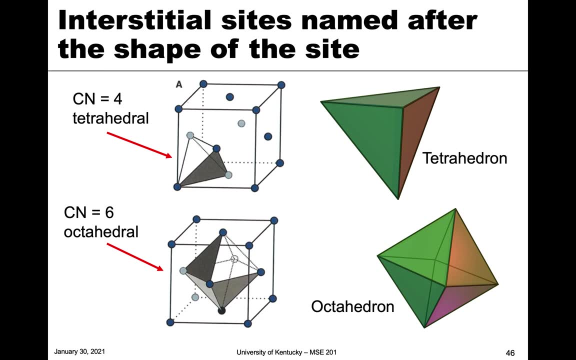 touching and close packed that we have just the FCC. But this is just a way of a schematic to think about the way these structures are built. Okay, so let's look at these interstitial sites. So these interstitial sites, So these are the ones for FCC. so 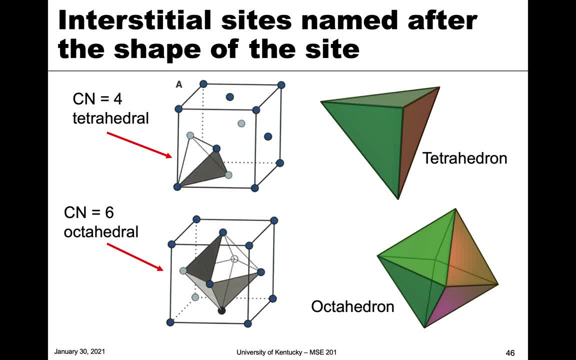 cubic They're named after, not the kind of where they're at, but the shape that it appears That these take. So if we look at the empty space here, so basically there's an empty space right in the middle, And so if we kind of draw lines connecting all the atoms that are around that space, 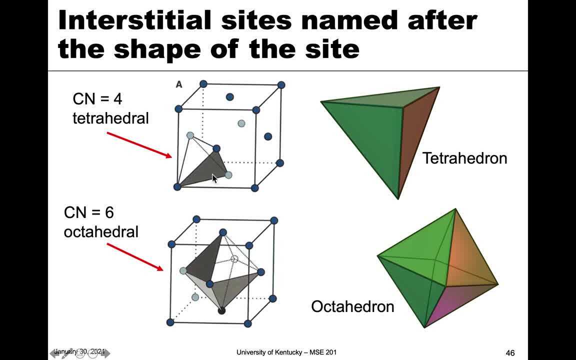 We get a tetrahedron, And so we call this space here that is surrounded by four atoms or ions. So coordination number four, We call this a tetrahedral. So even if you might think tetra as in three or so. 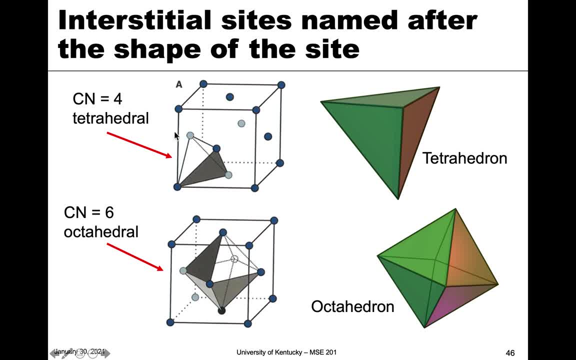 is totally fine because of the shape right, so it forms a tetrahedron shape, so we have six. and then the same thing here. if we look at the spot, there's a spot right in the middle of the cube and it's surrounded by six, if I keep my cursor back. 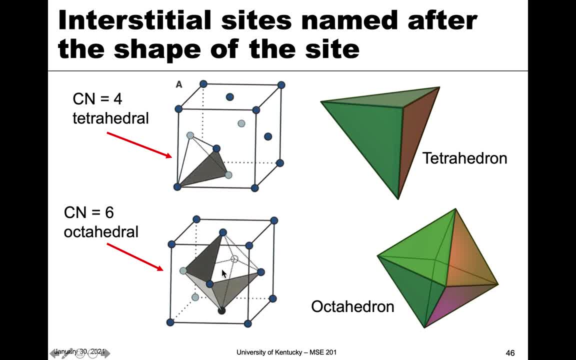 surrounded by six atoms around it, or ions, but it's not named for something that might make you think of six. it's actually octa, octahedral, because if you draw out the shape putting lines between all the, the, the atoms, here we get an octahedron, and so that's octahedral interstitial site. and so these are the. 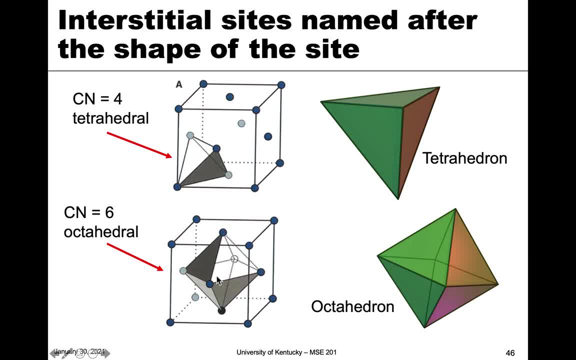 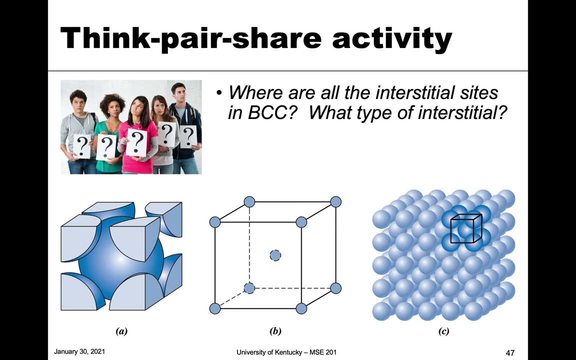 two different sites that we have and if you can kind of visualize them right here, relatively speaking this one is bigger than the tetrahedral, so octahedral is bigger than tetrahedral. okay, so that was FCC. so I mentioned that the anthropomorphic and ions form into one of the close packs. so FCC or HCP, but just you know. 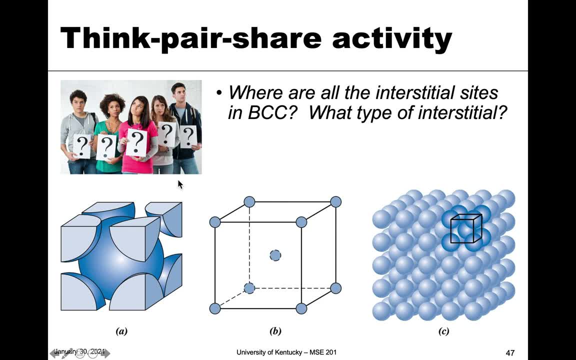 kind of bear with me here, just so we can kind of think about interstitials. let's think about BCC. so take the BCC structure that you see here, pause the video. let's see if you can kind of identify on any one of the structures. 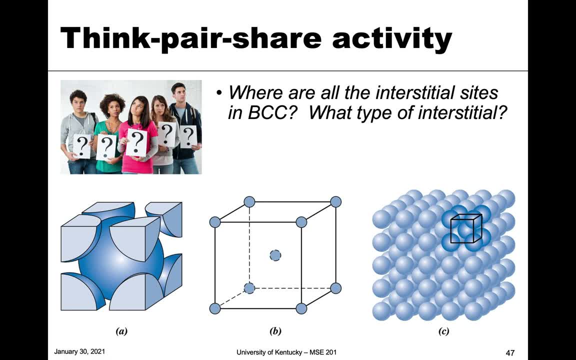 you want, but see if you can identify the interstitial sites in BCC and what type you know, for example tetrahedral or octahedral. so pause the video and see if you can find them and identify what type they are, and then we'll come. 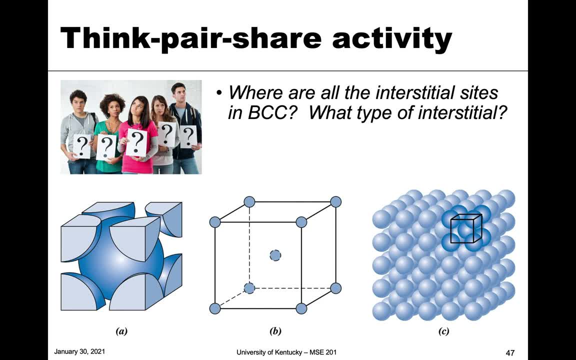 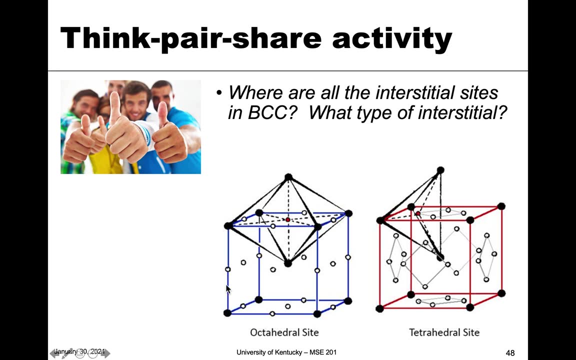 back and we will discuss all right. so let's go ahead and take a look at these interstitial sites in BCC again. keep in mind, this is like a side example. this doesn't have to do with ceramic structures, okay, and so here's a schematic showing you that there are both octahedral and tetrahedral sites in. 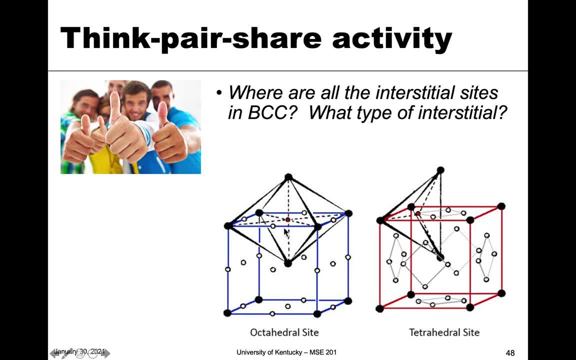 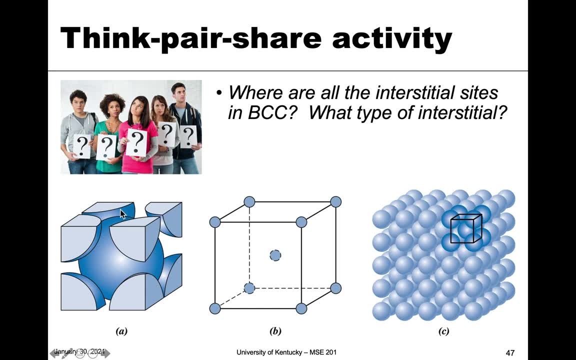 BCC. the octahedral are basically on the face centered positions. so if we go back it might be a little easier to tell. so right here on the face right there's an empty spot between all of these atoms. so that is an octahedral, because if we do, 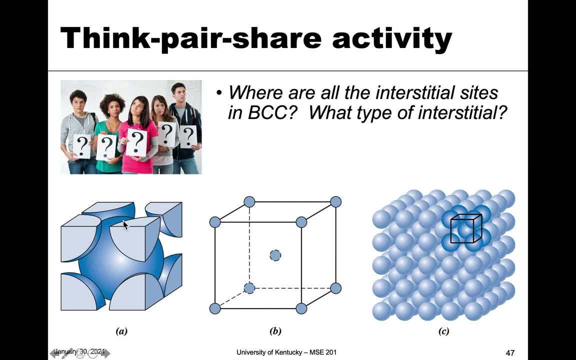 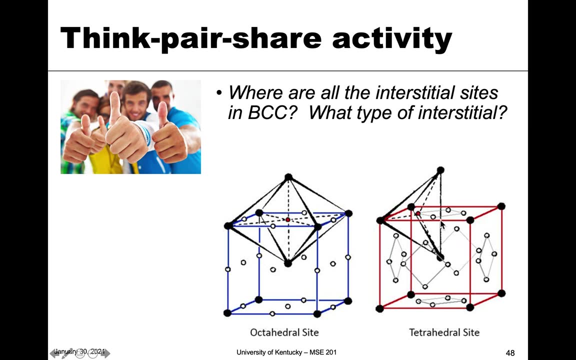 the count, then there's going to be four around it plus one below it, and if we look at the next unit cell above, there's going to be another body centered at them above it. so that's six. all right, so then there are also tetrahedral sites that we see, and those are you can see. 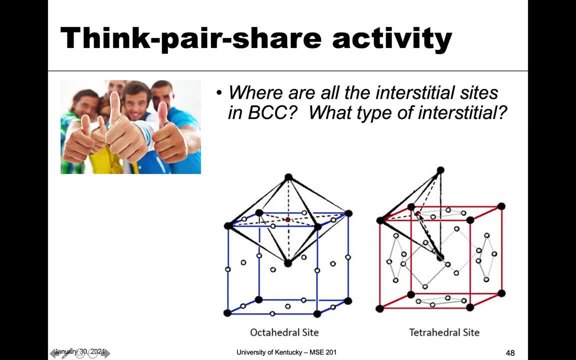 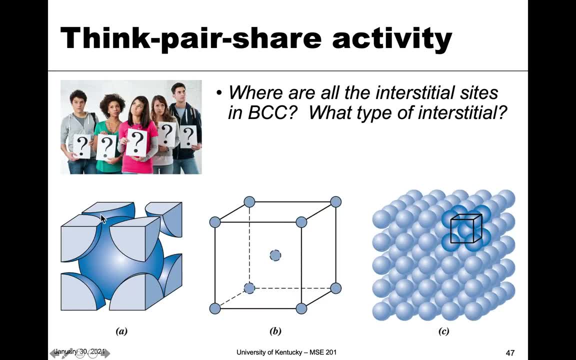 here as the red, so this type, and if we go back it might be a little easier to see. but basically, over here, right, there's also an empty spot between these two atoms and for these sites, again, there it's. it would be touching this one, this one and then the one below and then one above, so that.